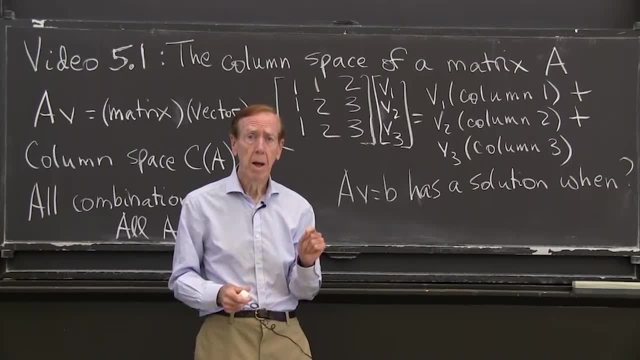 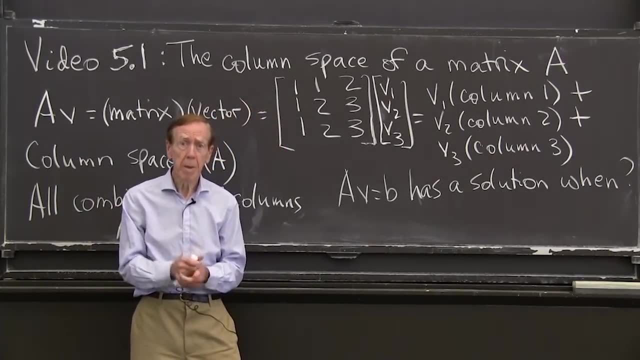 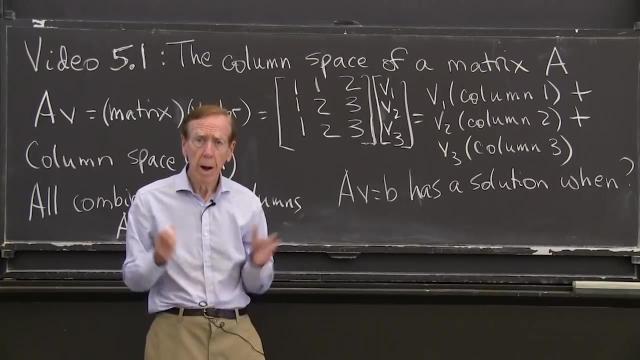 That would be available, you may know, on OpenCourseWare for 18.06.. That's the linear algebra course, But why not just say them here in a few minutes? So I have a matrix. Well, there's a matrix. 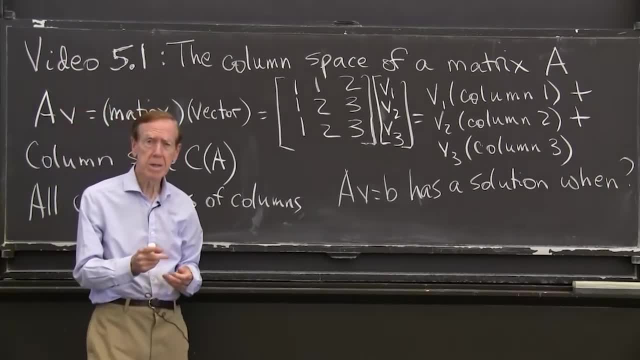 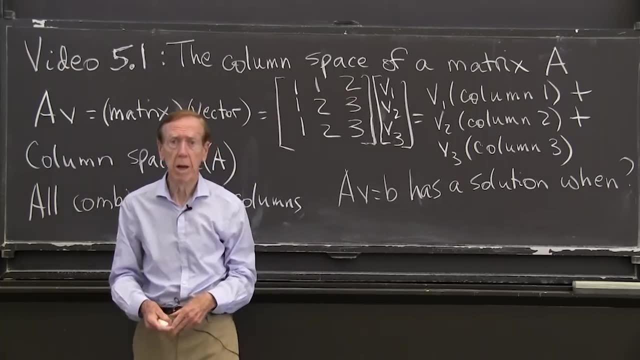 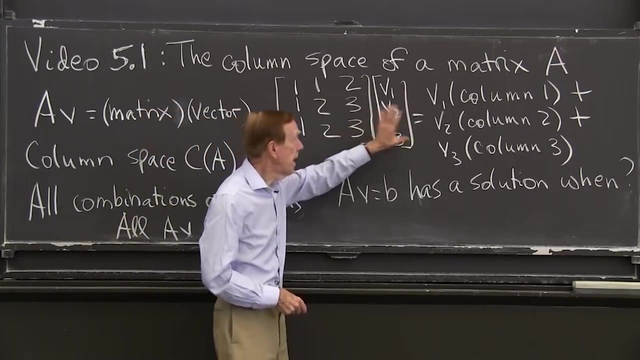 That's a 3 by 3 matrix. And first I want to ask: how does it multiply a vector? So there it is, multiplying a vector v1, v2, v3. And what's the result? Key idea: It takes the answer on the right-hand side. 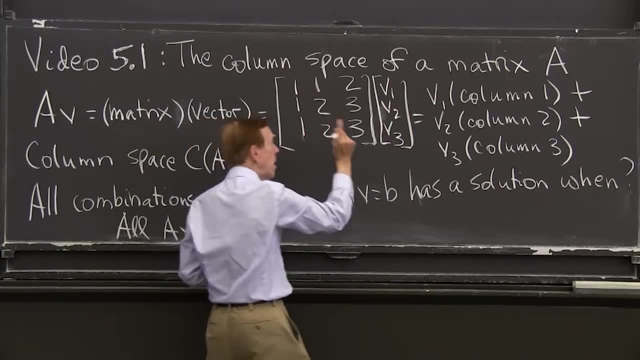 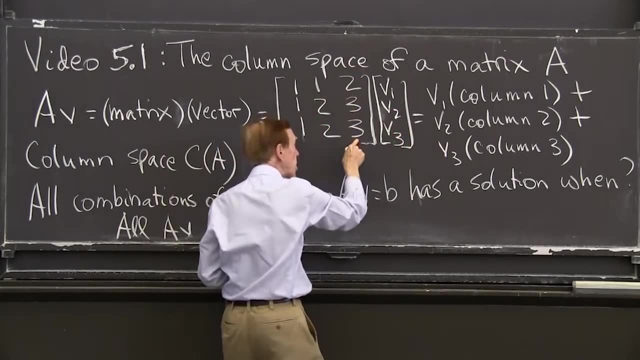 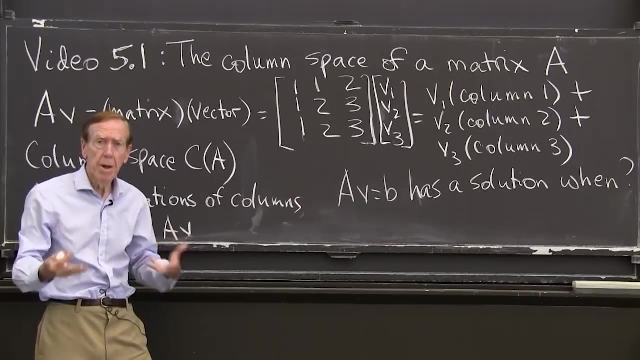 is this number: v1 times that column plus this number. that number times the second column plus the third number. the third number times the third column. Combination of the columns of A. That's what A times v is. That's what the notation of matrix multiplication produces. 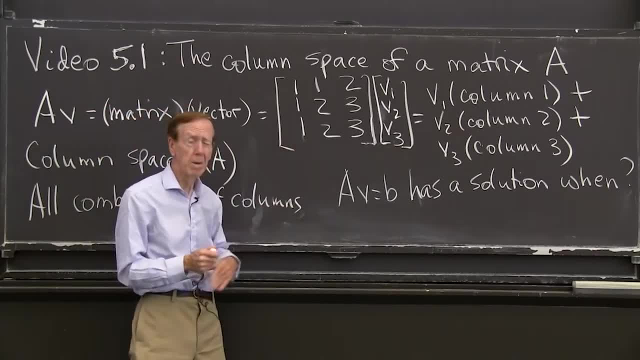 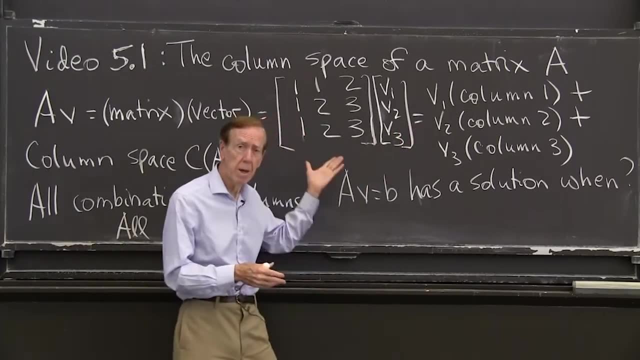 That's really basic, to see it as a combination of columns. Now I want to build on that. That's one particular. If you give me v1,, v2, and v3, I know how to multiply. I take the combination. 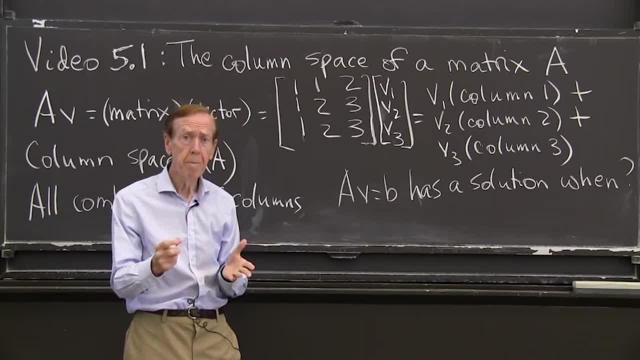 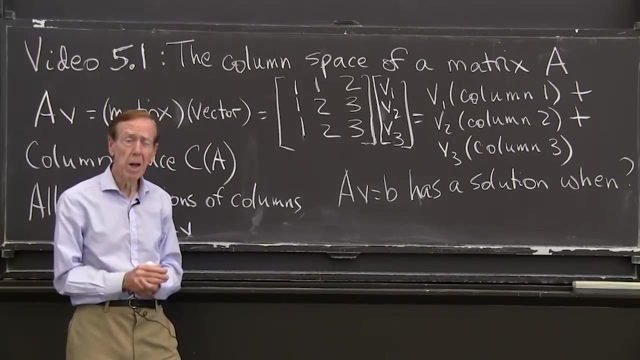 Now I would like you to think about the result from all v1,, v2, and v3.. If I take all those numbers then I get a whole lot of answers. They're all vectors. The result of A times v is another vector, Av. 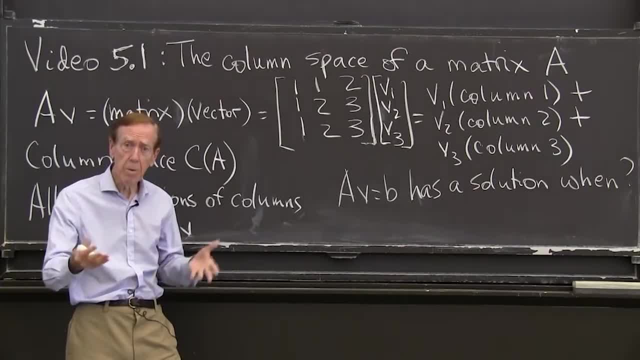 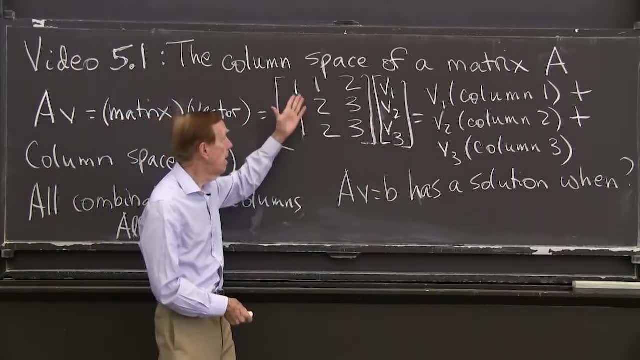 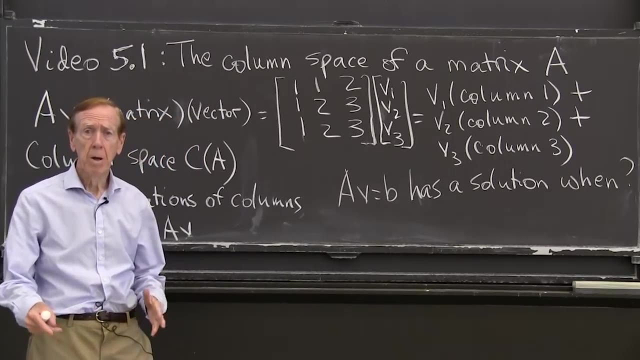 And I want to think about Av, those outputs, for all inputs v. So I take v1, v2, v3 to be numbers And I get all combinations of those three columns And usually I would get the whole three-dimensional space. 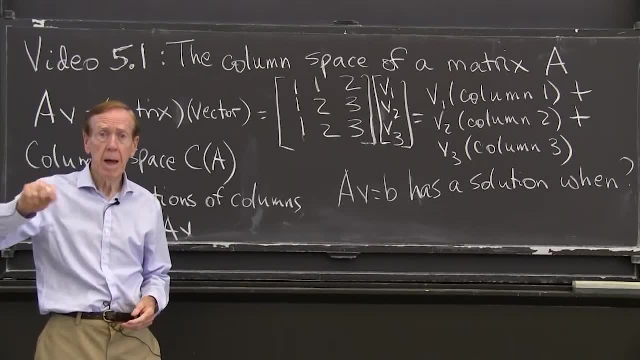 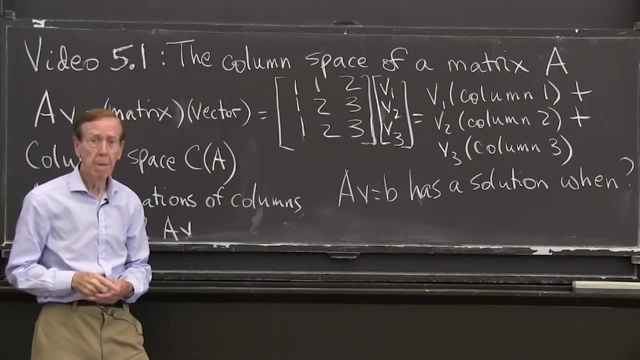 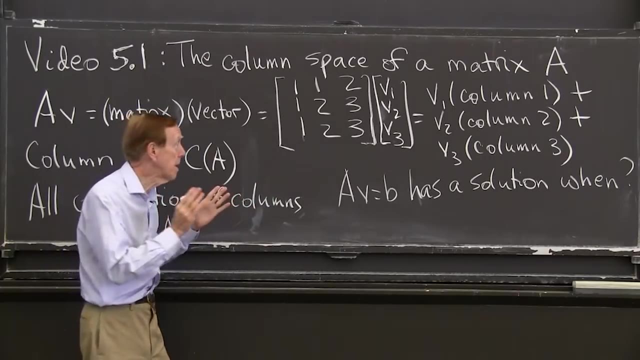 Usually I can produce any vector, any output- v1,, v2,, v3, from A times v, But not for this matrix. Not for this matrix because this matrix is, you could say, deficient. That third column there, 2, 3,, 3, is obviously. 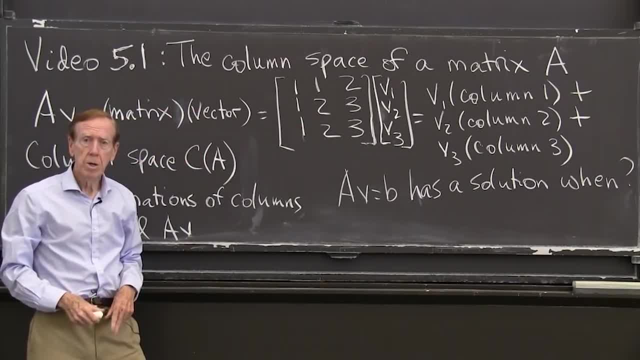 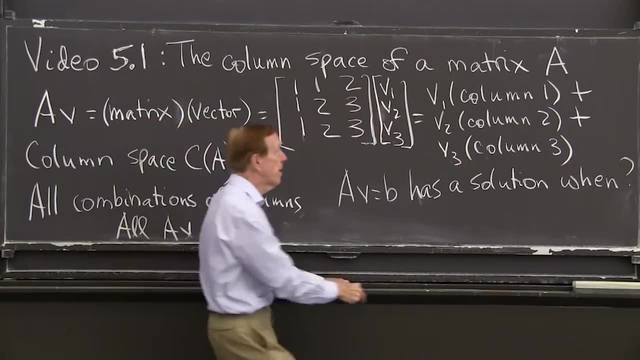 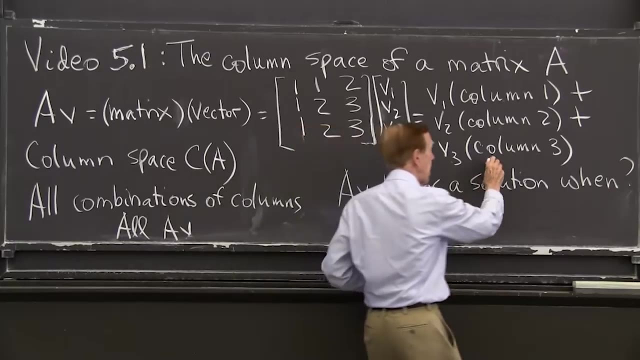 the sum of columns 1 and column 2.. So this v3., v3. v3. v3. v3 times that third column just produces something that I could already get from column 1 and column 2. That v3 times column 3, that column 3, I could x out. 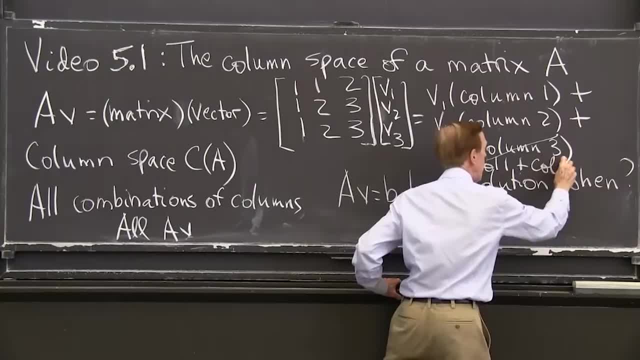 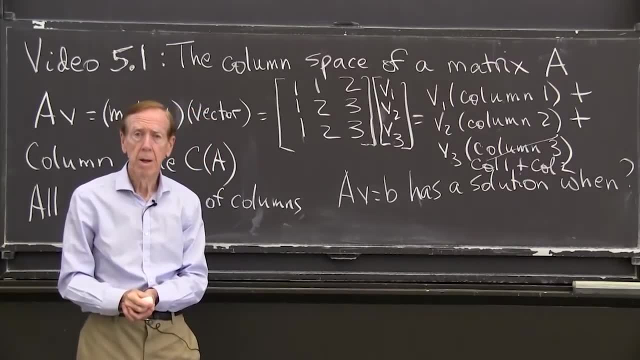 That's the same as column 1 plus column 2 for this matrix- Not usually, And then so I only really have a combination of two columns. It's a combination of three, but the third one was dependent on the others and it's really a combination. 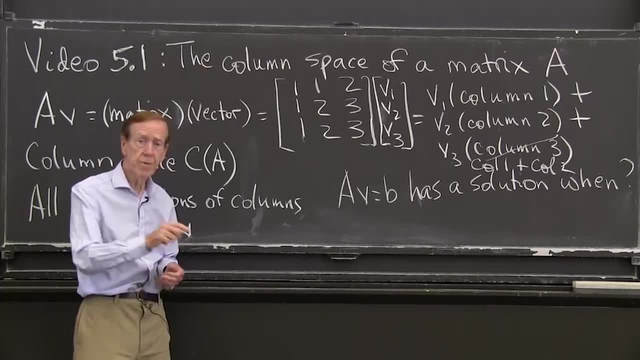 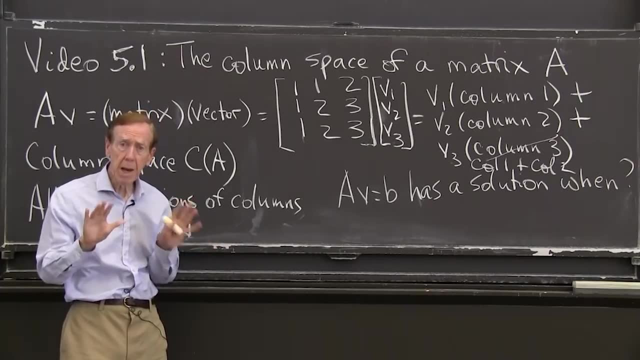 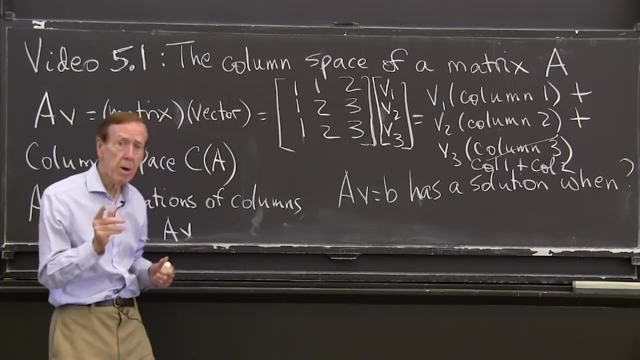 of two columns. So combinations of two columns, two vectors in three-dimensional space produce a plane. I only get a plane Now. I don't get all of three-dimensional space, only a plane, And I call that plane the column space. 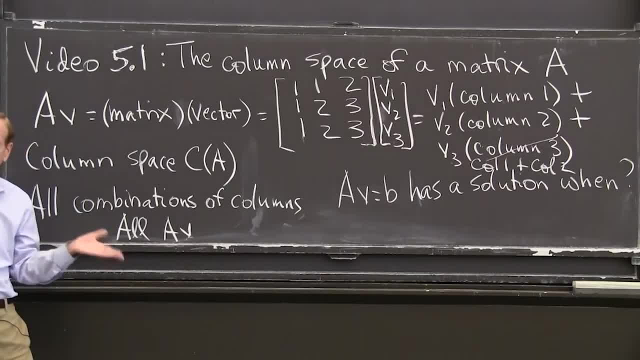 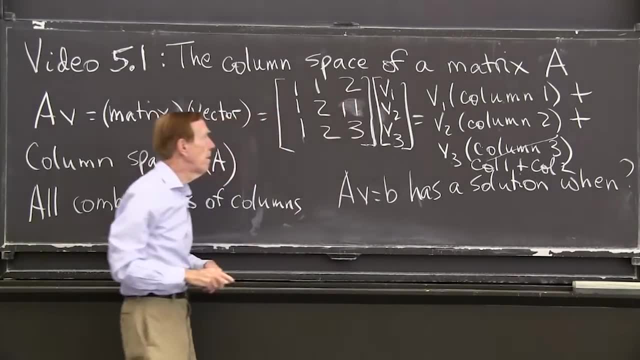 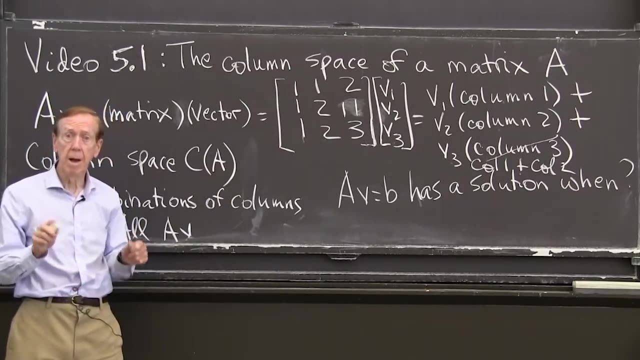 So the column space of the matrix. So if you gave me a different matrix, if you change this 3 to 11, probably the column space now changes to. for that matrix I think the column space would be the whole three-dimensional space. 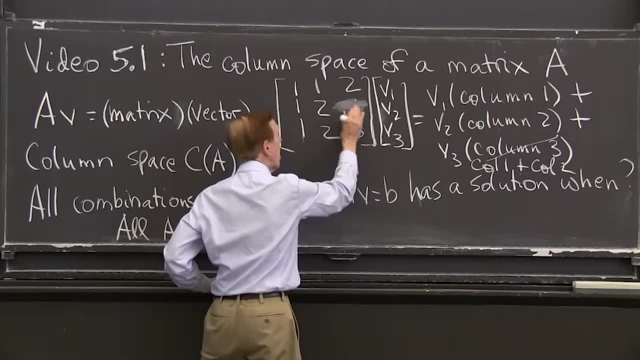 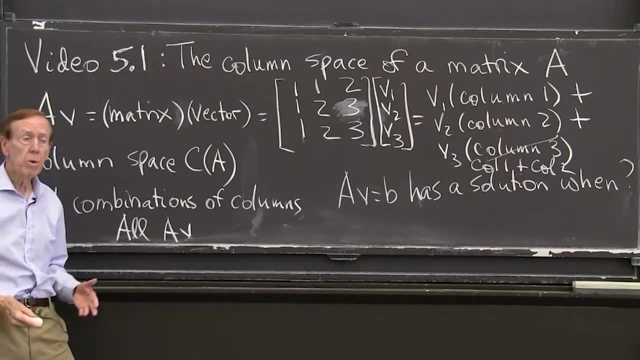 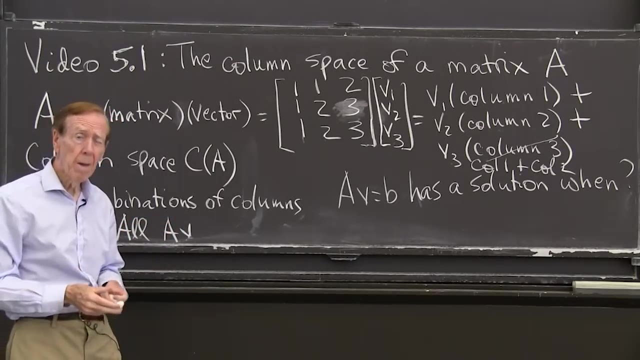 I get everything, But when this third column is the sum of the four columns, it's not giving me anything new. and the column space is only a plane. And you could think of a matrix where the column space is only a line, just one independent column. 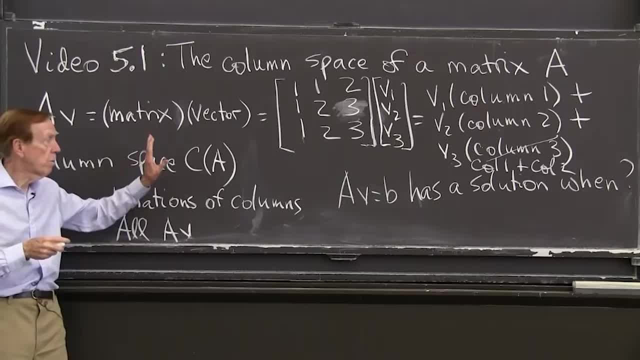 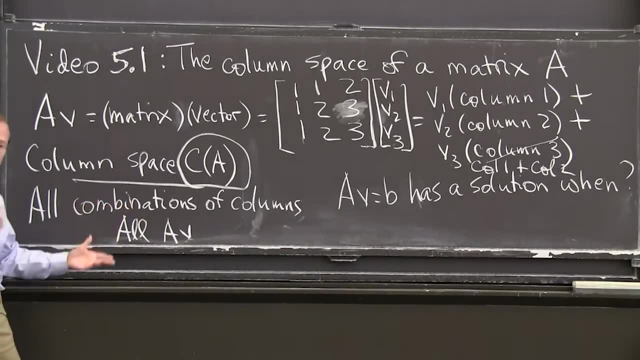 OK, so we thought about, this is all combinations of the columns. In other words, it's all the results, all the outputs from A times V. It's all the outputs from A times V. Those are the combinations of the columns. 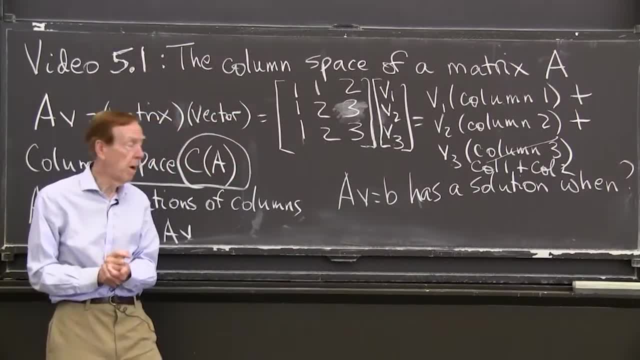 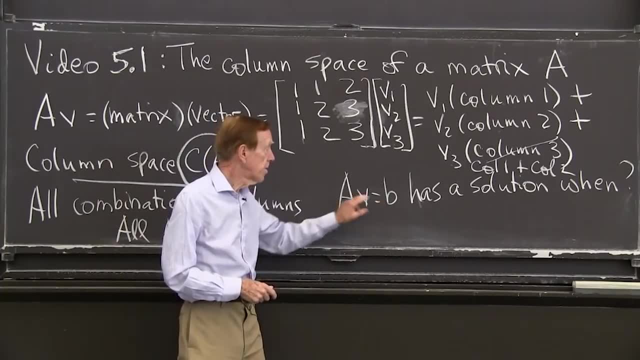 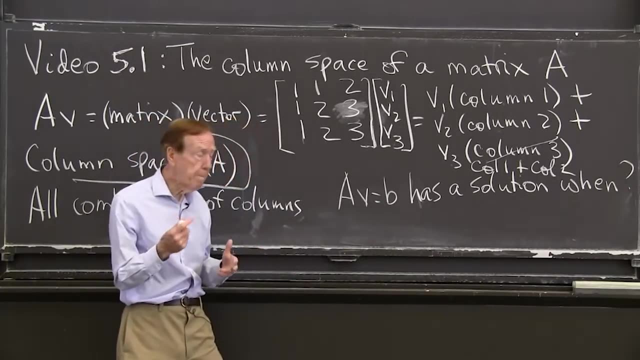 So we can answer the most basic question of linear algebra: When does A V equal B have a solution? When is there a V so that I can solve this? When is there a V that solves this equation? So it's a question about B. What is it about B? that must be true. 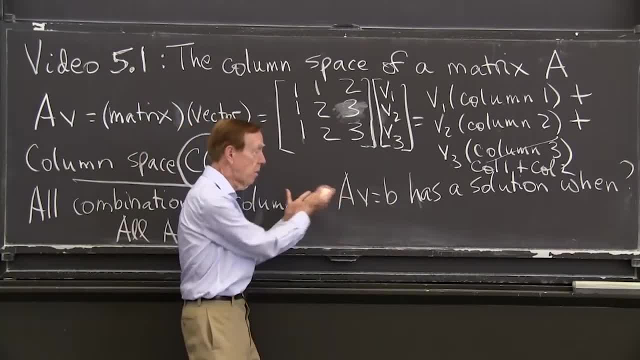 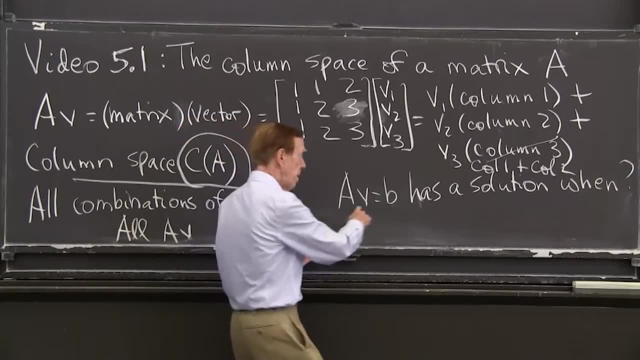 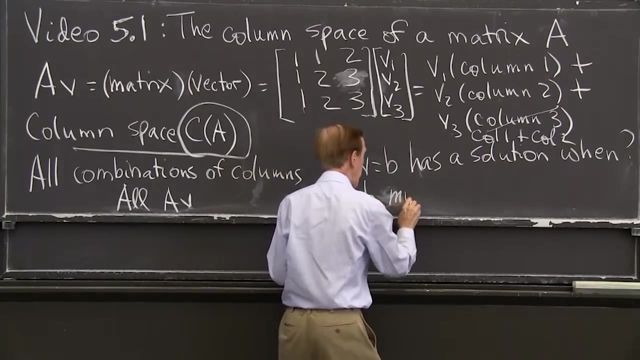 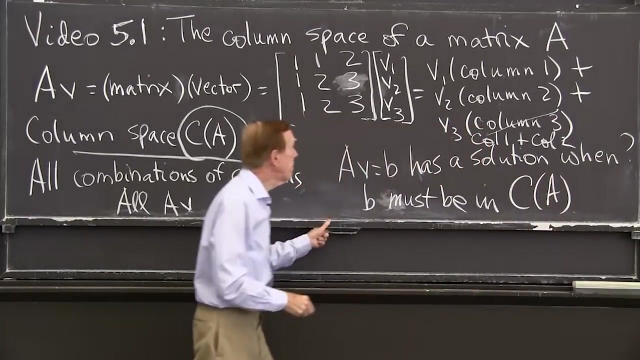 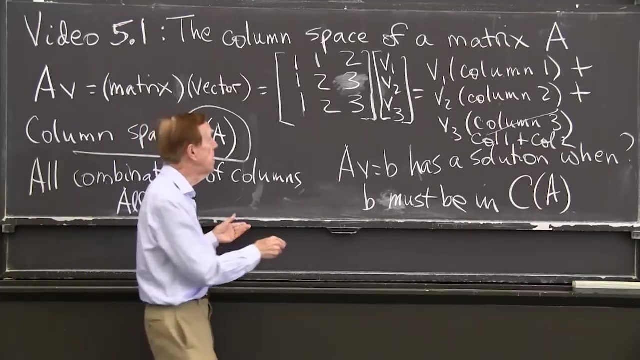 if this can be solved. Well, this says that equation is saying: B is a combination of the columns of A, So this has a solution. when B is me must be- shall I say, must be- in the column space For that example, only B's where we can get a solution. 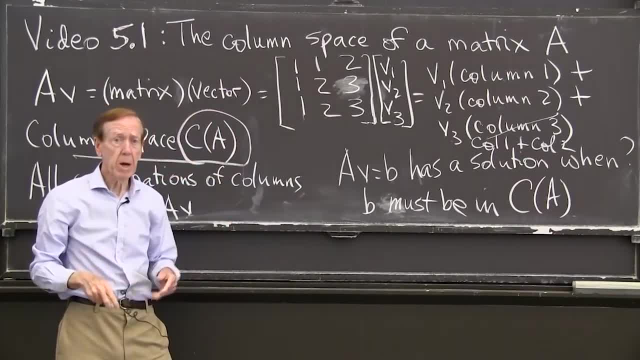 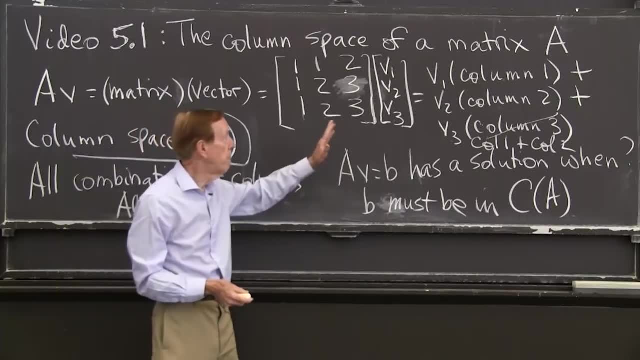 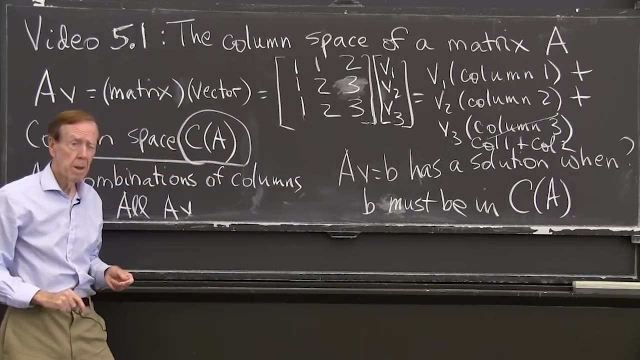 B's that are combinations of the first two columns, Because having the third column at our disposal gives us no help, doesn't give us anything new. It would be solvable if B equal 1, 1, 1.. That's a combination of the columns. 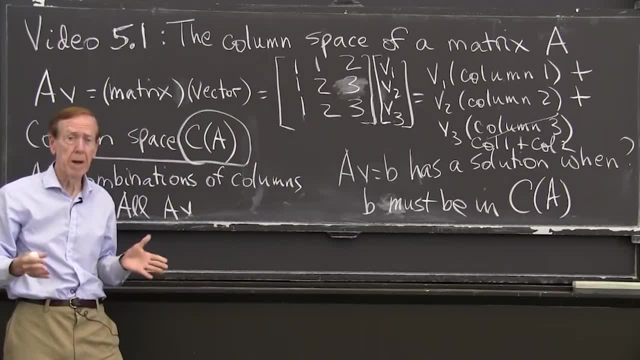 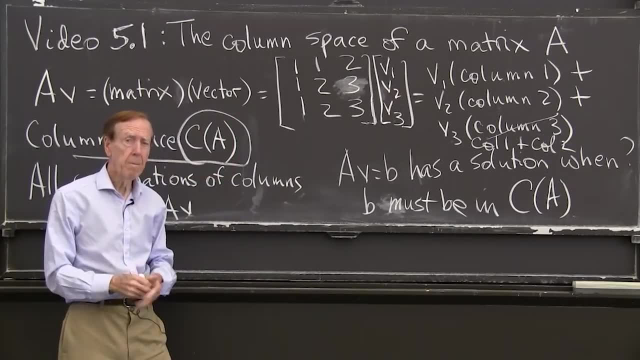 Or if B equals 1,, 2, 2.. That's another simple combination of the columns. Or if B equals 2,, 3, 3.. But I'm staying on a plane there and most B's are off that plane. 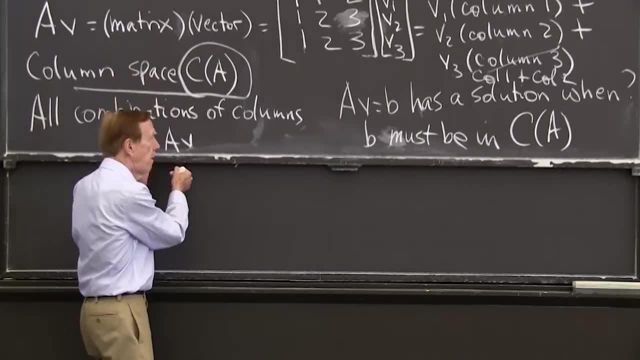 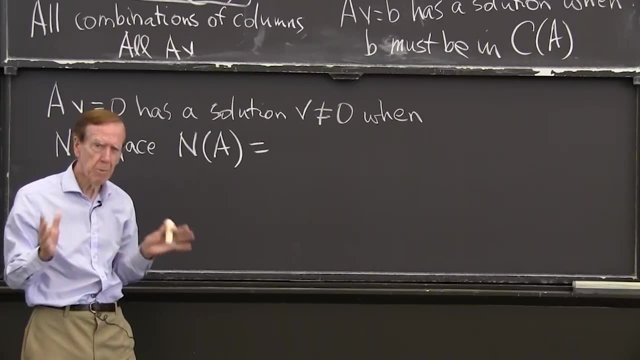 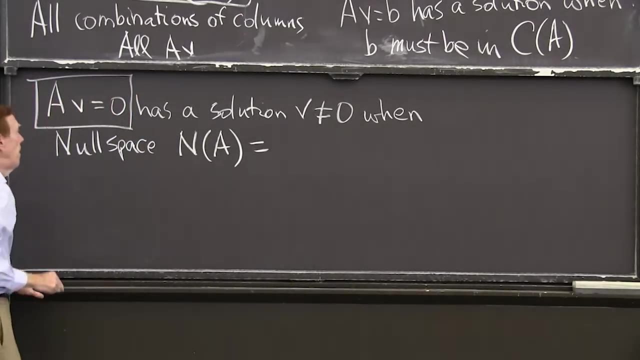 Now there's a solution, All right Now. Now A second, A second. This is a key idea of linear algebra. Can we do it in this short video? I want to know about the equation B equals 0.. So now I'm setting the right-hand side to be 0.. 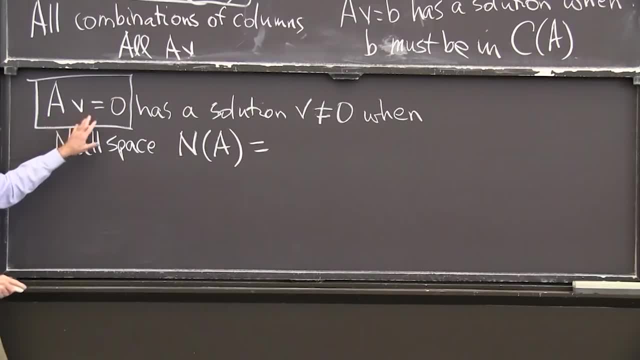 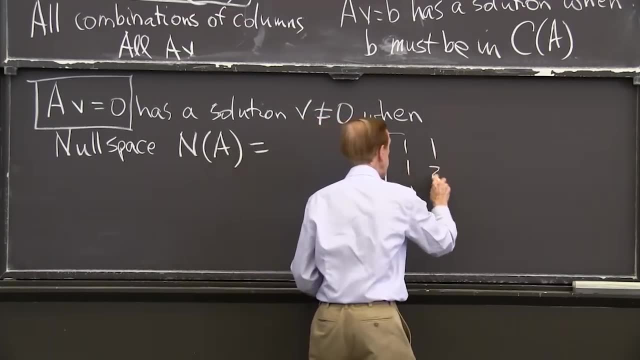 That's the 0 vector: 0, 0, 0.. Does it have a solution? Does it have a solution? Let's take this example: 1, 1, 1, 1, 2, 2, 2,, 3, 3.. 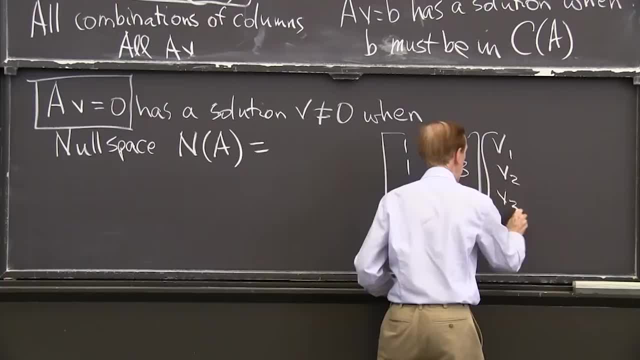 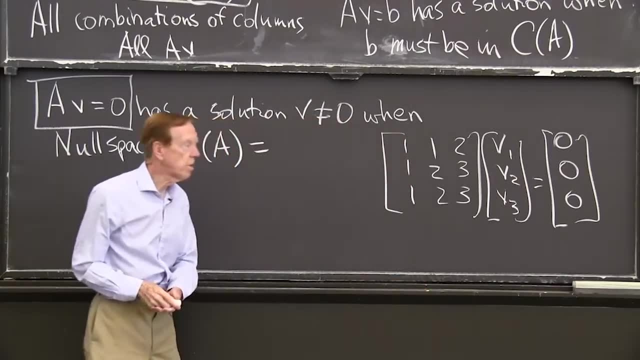 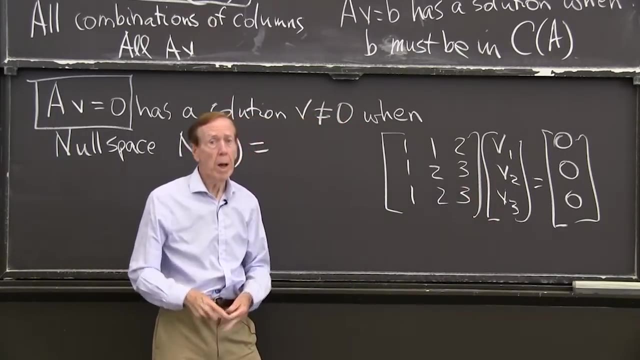 Now- Now I'm looking at the solutions- when the right side is all 0. Does that have a solution? Is there a combination of those three columns that gives 0?? Well, there is always one combination. I could take 0,, 0, and 0. 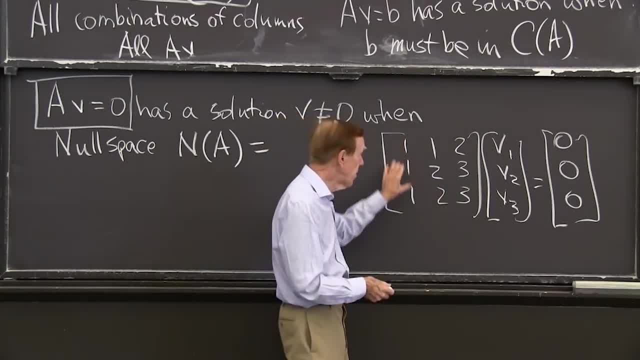 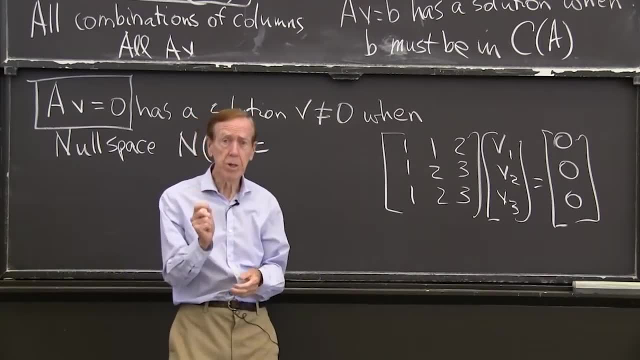 I could take nothing. 0 of everything. 0 of this column, 0 of that column, 0 of the third column would give me the 0. That solution's always available. The big question is: is there another solution? 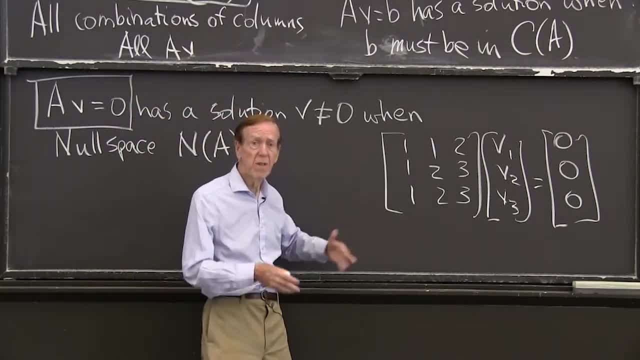 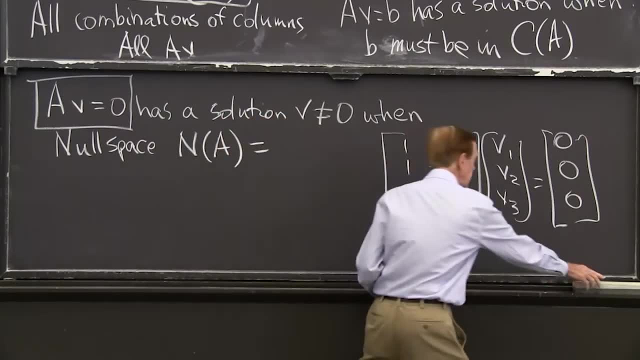 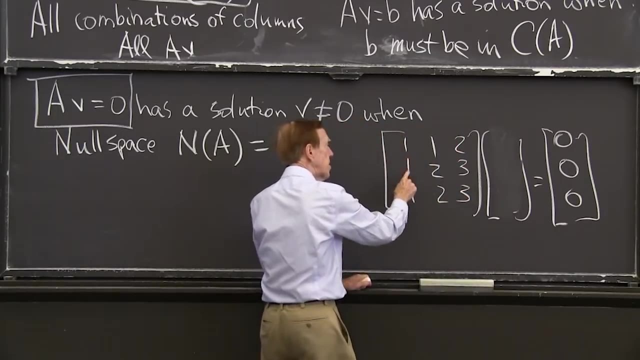 And here, for this deficient, singular, non-invertible matrix, there is. There is another solution. Let me just write it down. Let me put it in there. Do you see what the solution is? This column is the sum of those two. 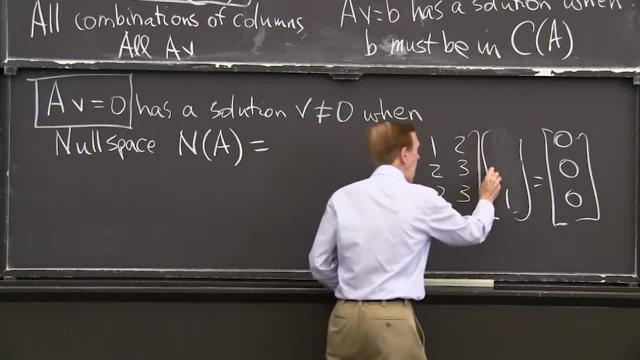 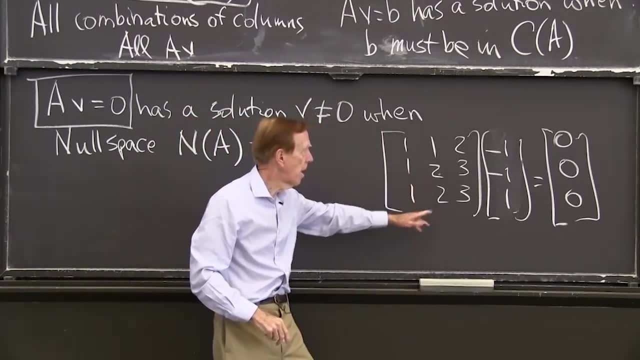 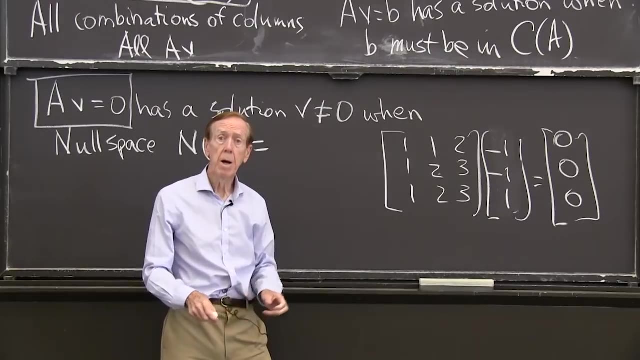 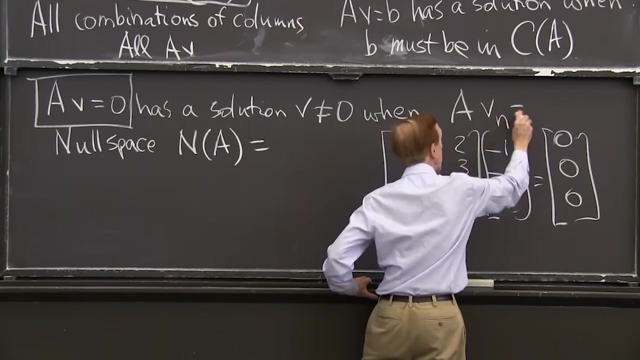 So if I want one of that, I should take minus one of the other columns. So this is minus this column. minus this column. plus this column gives me the 0 column. That is a vector in the null space. That's a solution to a v? n equal to 0.. 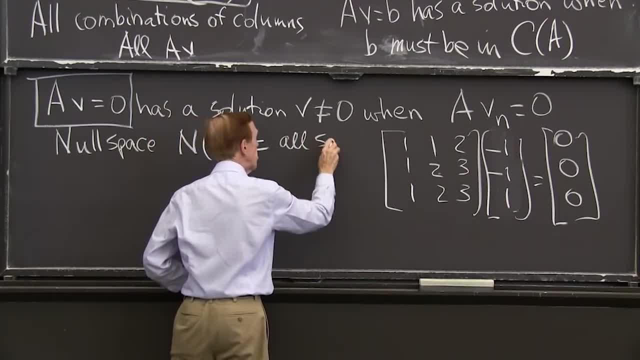 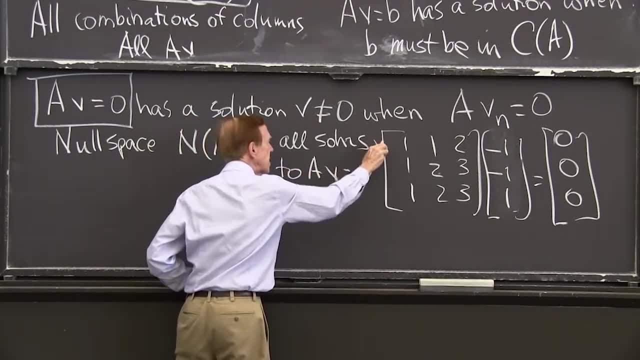 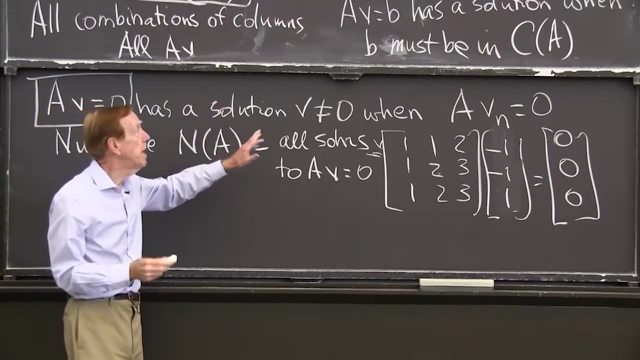 So the null space is all solutions to a v n equal to 0. It's all the v's. The null space is a bunch of v's. The column space was a bunch of b's. Can I just emphasize that difference? 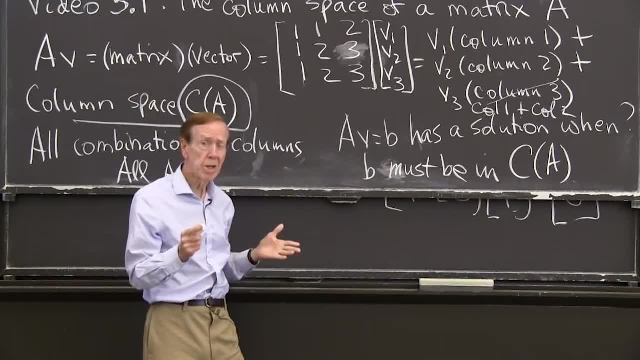 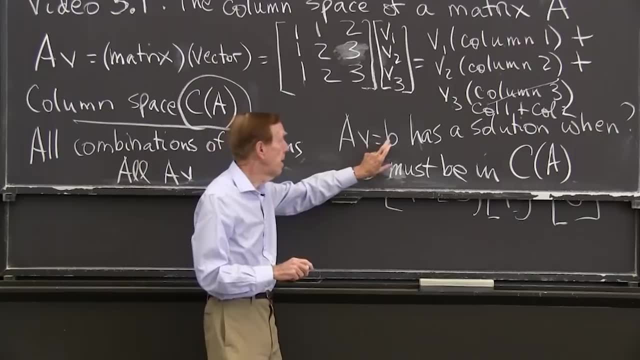 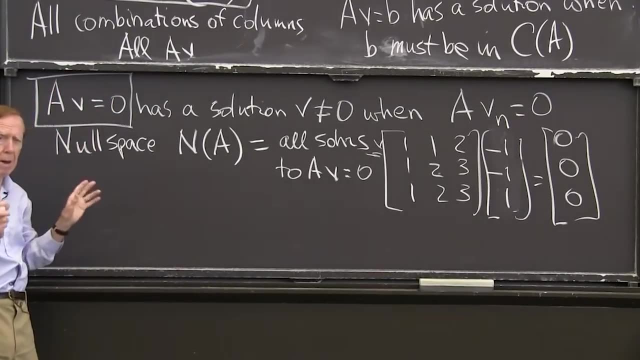 I was looking at which b. I wasn't paying attention to what that solution was Just. is there a solution? Then? that b is in the column space. I take. b equals 0. I fix that all important b, And now I'm looking at the solutions. 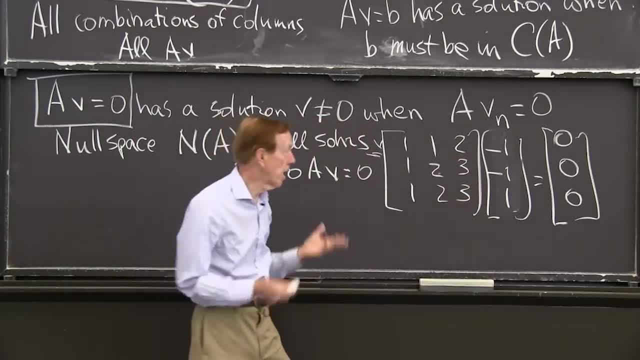 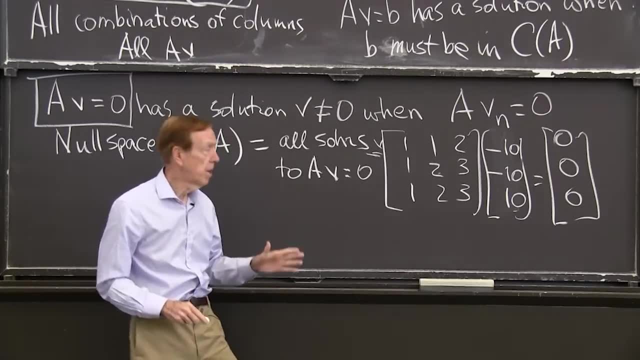 And here I find one. Can you find any more solutions? I think minus 10,, minus 10, and 10 would be another solution. It's times as much, And 0, 0, 0 is a solution. I think of solutions. 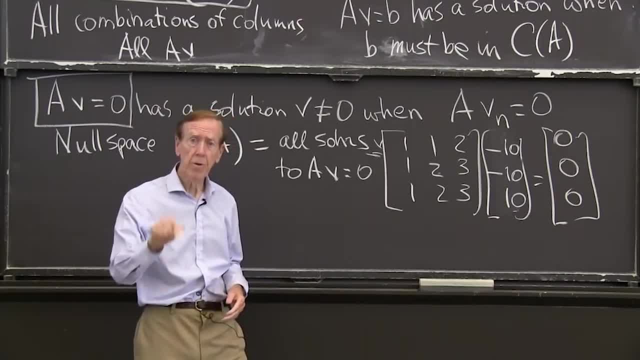 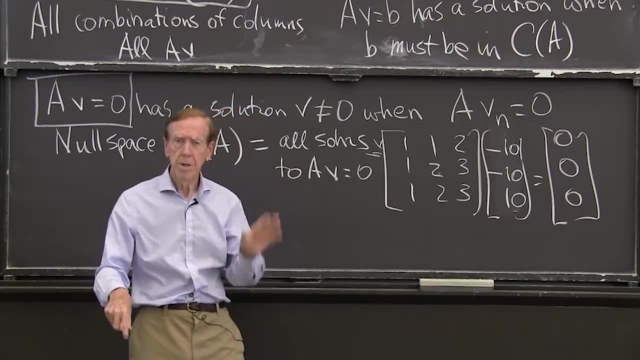 We had a plane for the column space, but we have a line For the null space. Isn't that neat. One's a plane, one's a line: Dimension two plus dimension one. Two for the plane, one for the line. 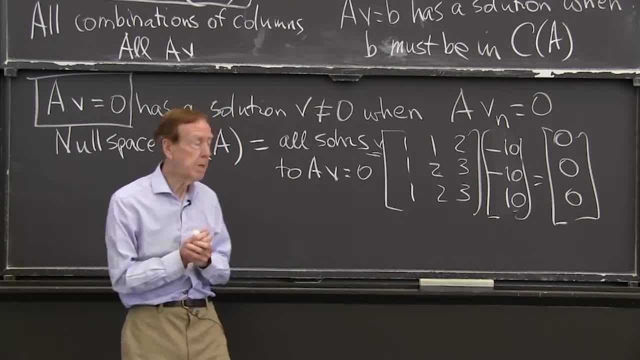 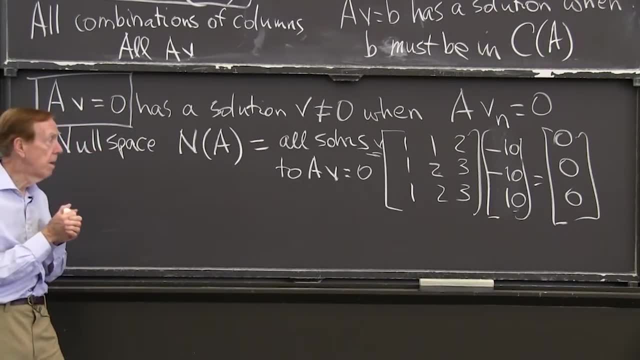 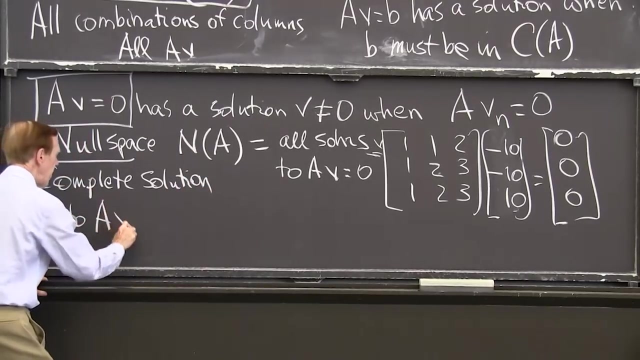 Adds to dimension three the dimension of the whole space. OK, that's a little going it All right. now I ask: what are all solutions? The complete solution To a v equals 12.. Let me choose some right hand side. 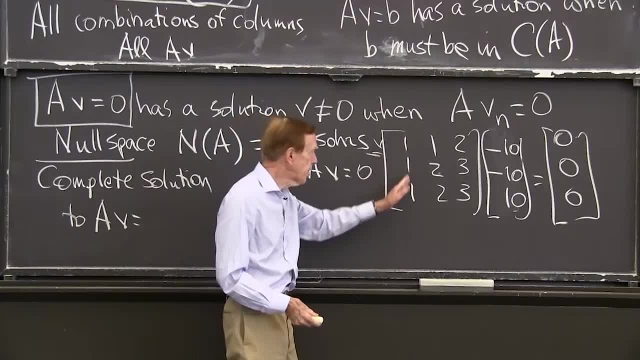 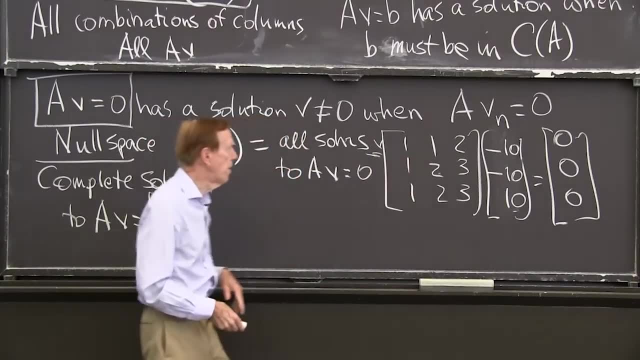 where there is a solution. Let me choose a right hand side, Say, if I add that column and that column I'll get a v. Or maybe I'll take two of that column plus one of that column. Two of the first column plus one of the second would be a three. 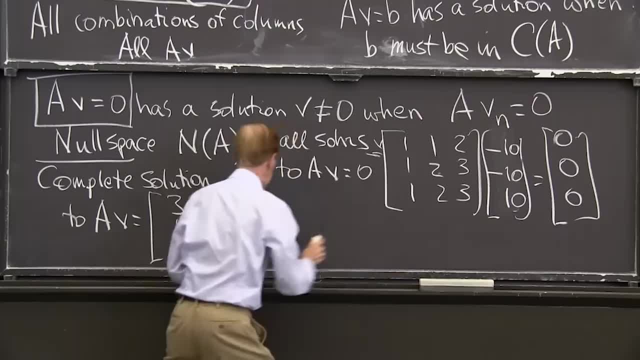 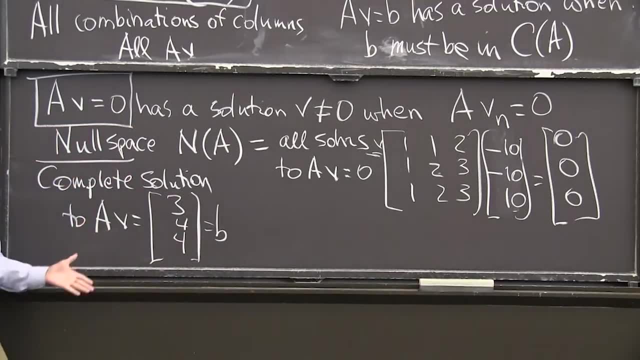 Two plus that would be a four. Two plus that would be another four. OK, OK, That's my b. It's a combination of columns. You saw me create it from the first two columns, So now I ask: what are all the solutions? 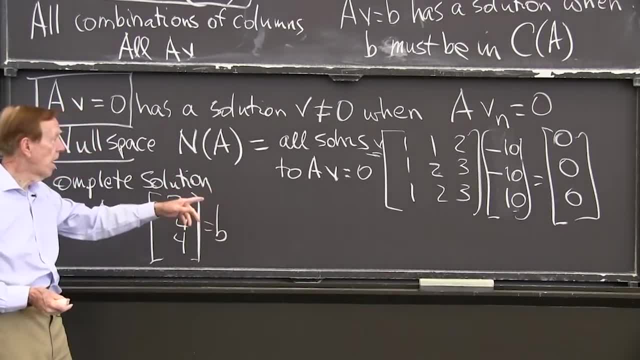 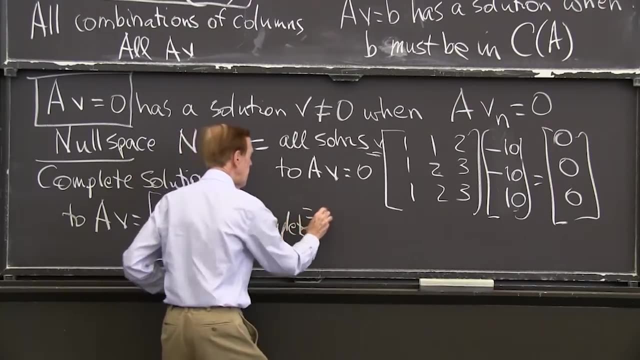 It's in the column space. It's two times the first column plus the second column. But there may be other solutions. So all solutions, A complete solution, V- complete. Here's the key idea, And the point is that it's the same that we 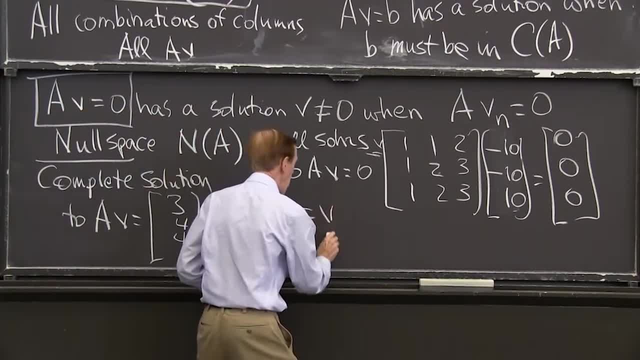 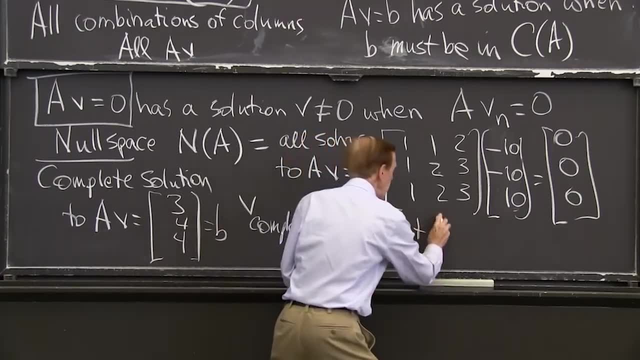 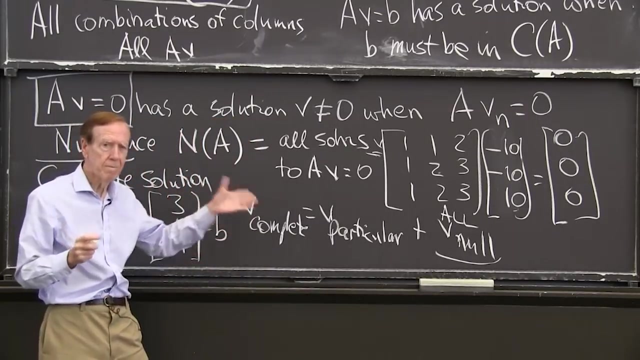 know from differential equations, It's one solution plus any null solution Plus all. You could say all v, null Particular plus null solution. OK, It's such an important concept, we just want to see it again. One particular solution with that thing. 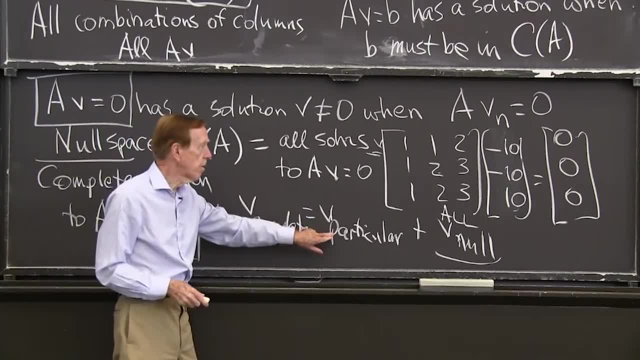 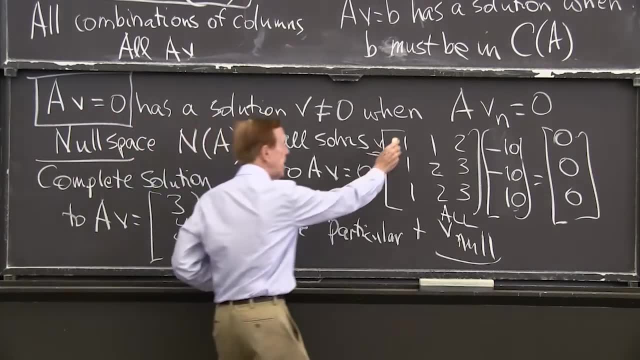 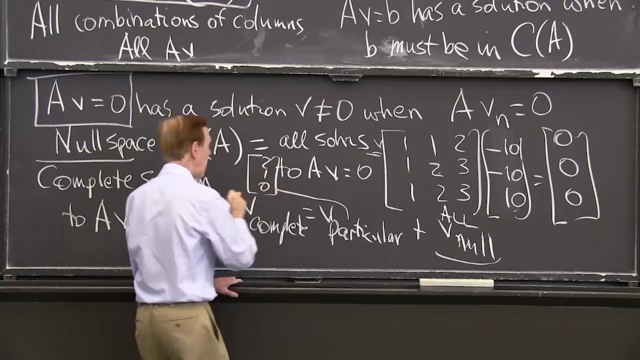 would be particular. v particular could be two. So how did we produce that Out of two of these plus one of these, plus zero of that? So v particular could be 2, 1, 0. It works for that particular b. 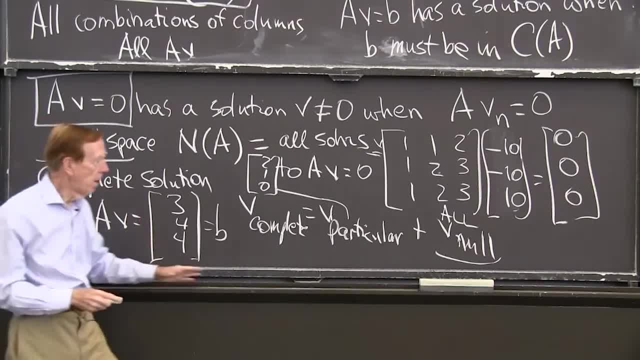 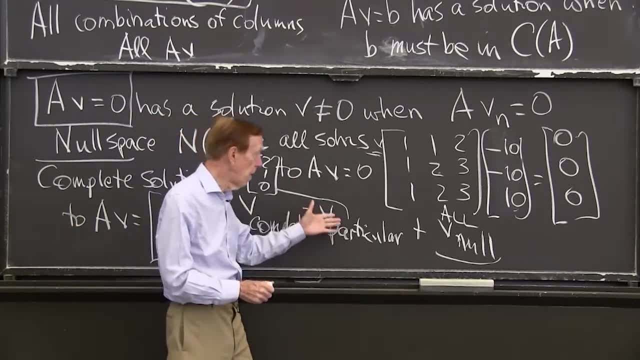 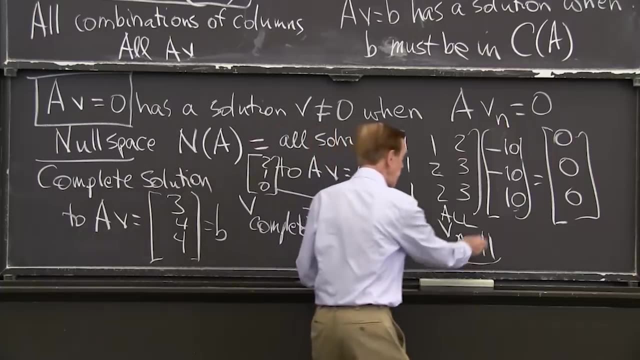 Two of the first column, One of the second. Now then we could add in anything in the null space. So we have infinitely many solutions here. We've got one solution plus, added to that a whole line of solutions. All the null space would be all vectors like that.